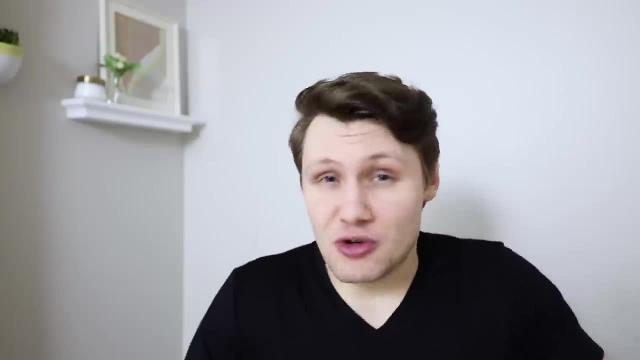 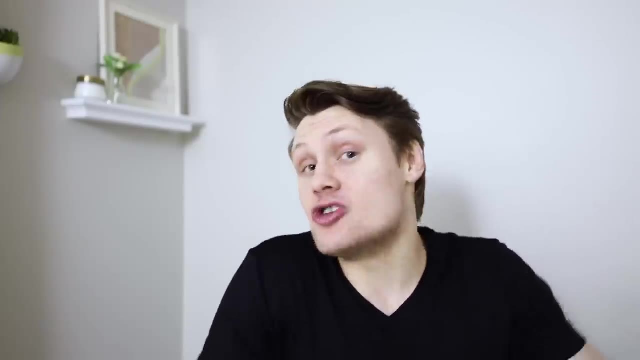 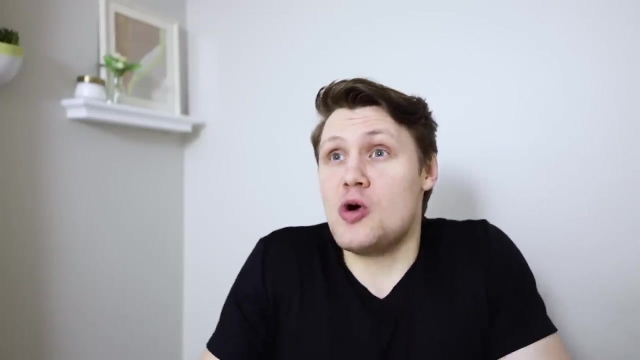 worse as a code reviewer to have to review 1000 or 2000 lines of code. And because reviewing that much code is difficult, it means that it's easier for a bug to introduce itself in the pull request and into the main repository eventually. Then the second reason is that it also makes it easier for 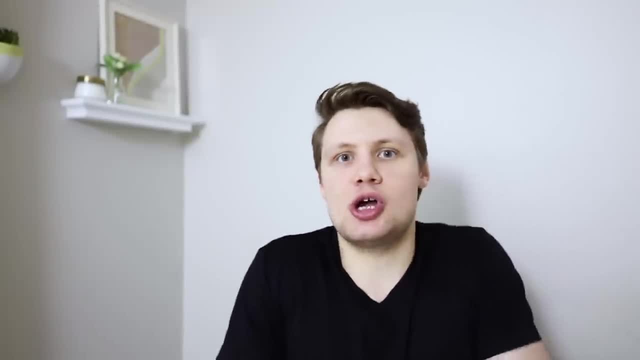 there to be a bug in the pull request to begin with because there's just a larger surface area of the pull request. And then the second reason is that it also makes it easier for there to be a bug in the pull request to begin with because there's just a larger surface area of code. And 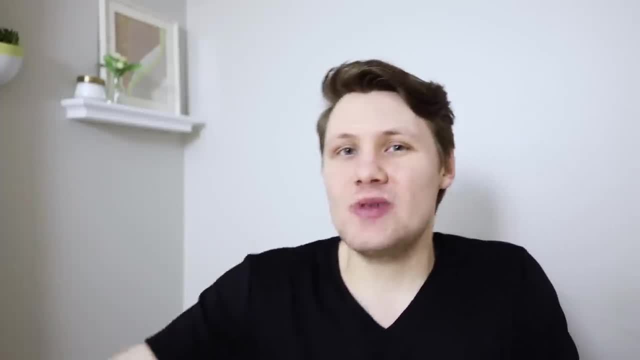 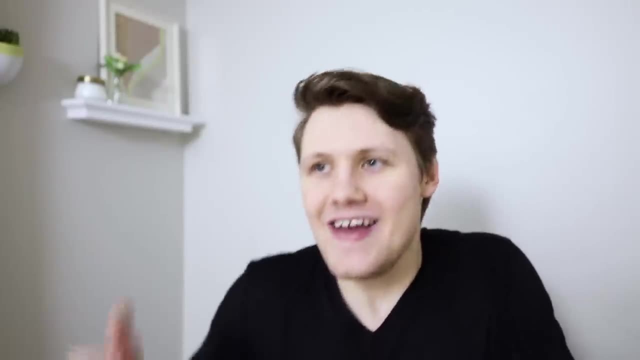 then, finally, it makes it much harder if you eventually have to revert the pull request because there was some bug that made its way into the main code repository. It's going to make it much harder because the more code you have in a pull request, the more likely it is that there's 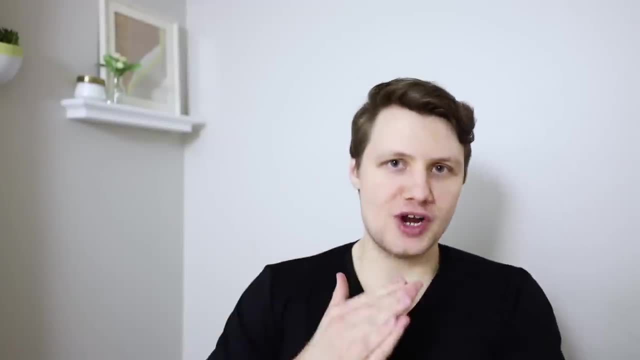 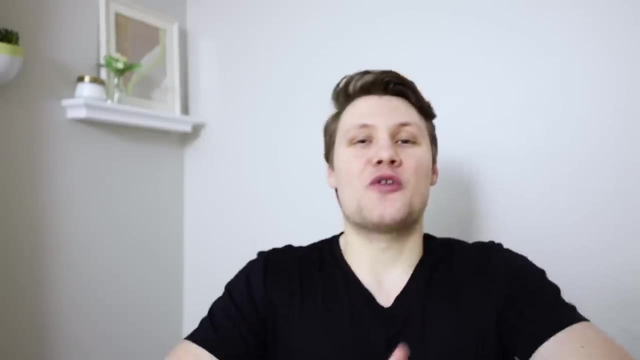 going to be a merge conflict with that pull request if you try to revert it And that's going to be just a nightmare. This is especially relevant if you work at a big tech company like Google or Facebook, where there are thousands upon thousands of engineers working on the 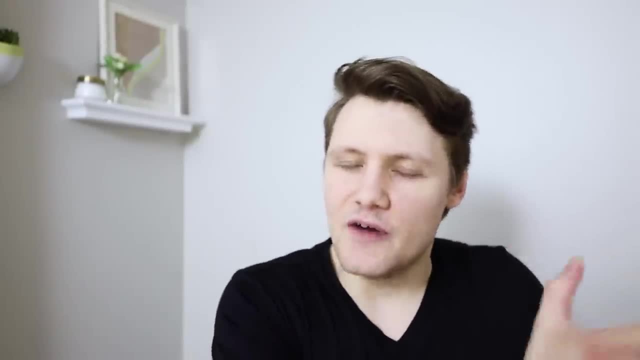 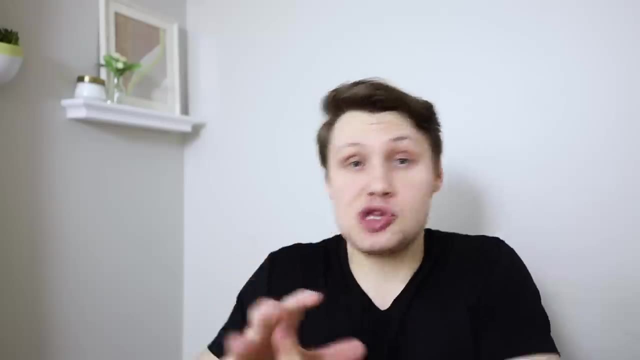 same code repository. So do try to err on the side of smaller pull requests. That might mean that you have to put in a bit more effort as the person writing the code, because you'll have to split up your code- let's say, if you're working on a big feature- into pieces that can be split up into. 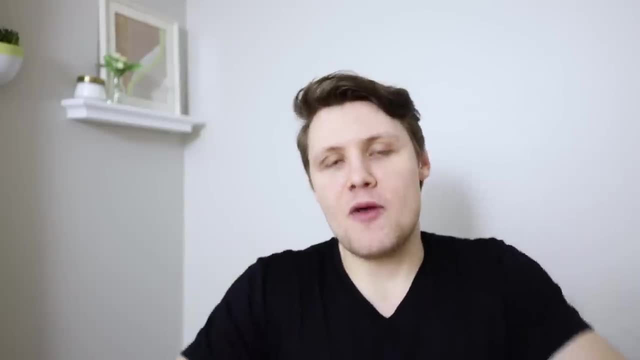 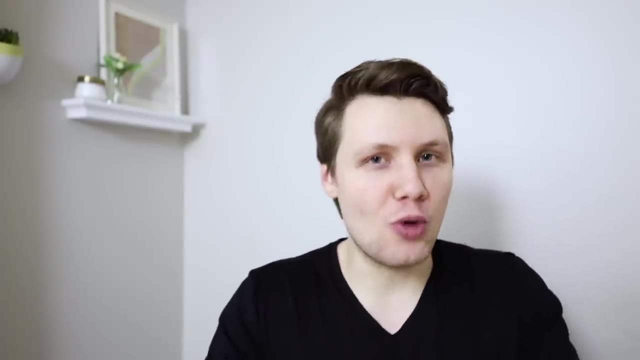 separate pull requests, But it will go a long way to make the entire software development process better. Software engineering best practice number two: This one also has to do with pull requests. When you're sending out a pull request, you ideally want to make sure that the pull request is. 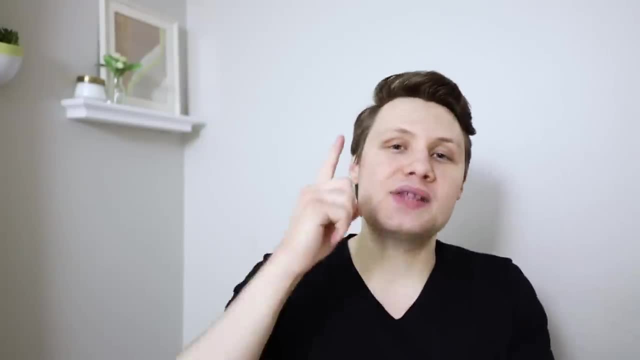 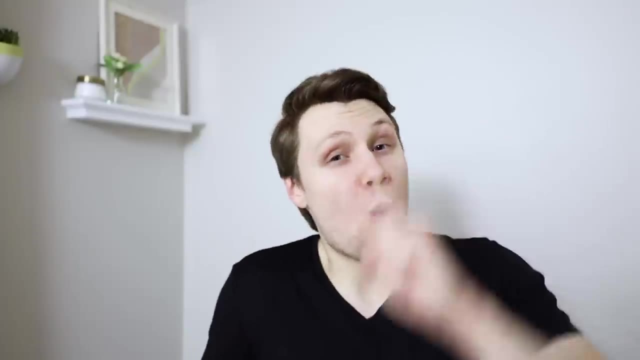 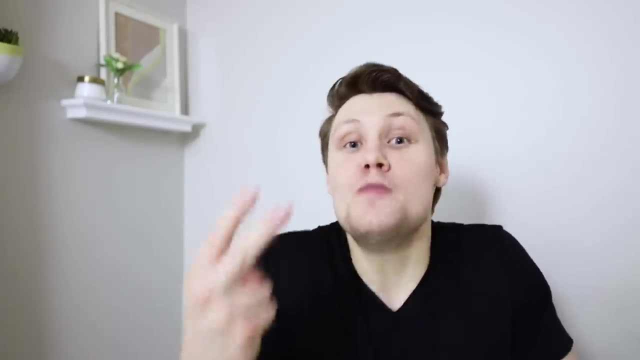 a single logical unit of code. What I mean by that is, if you're fixing a bunch of bugs, fix one bug in your pull request, Not two, not three, not ten. one bug, Unless you can fix, let's say, two bugs with one line of code, like the same line of code happens to fix two bugs. 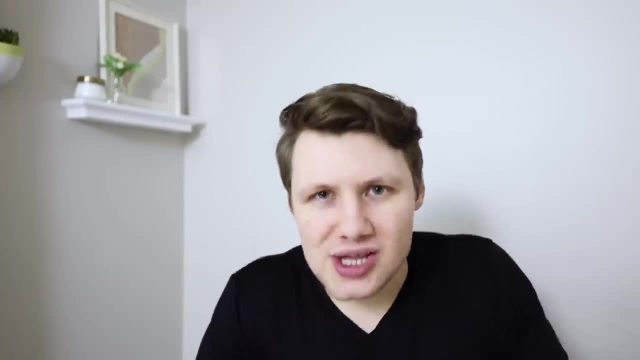 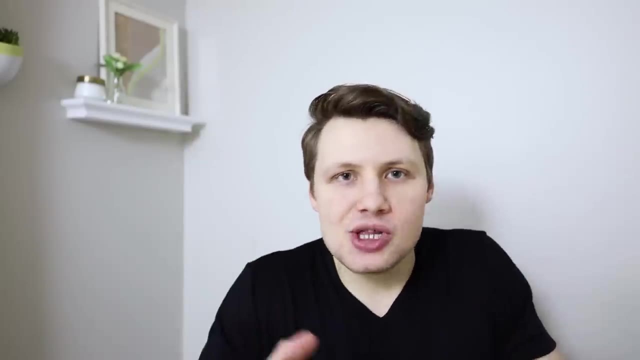 then that's fine, But otherwise limit each pull request to a single logical thing. The reasoning here is very similar to that first best practice. You want to minimize whatever a pull request is doing so that your code reviewer has an easier job reviewing it, so that you minimize the chance of introducing 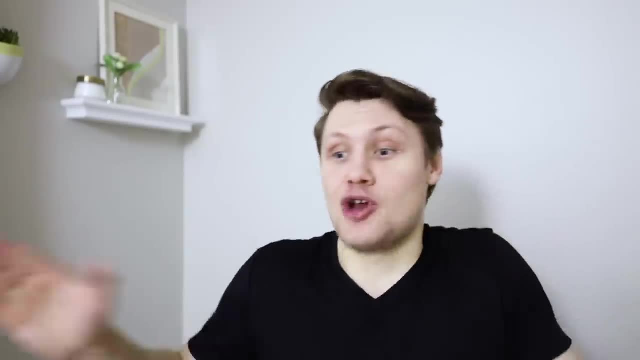 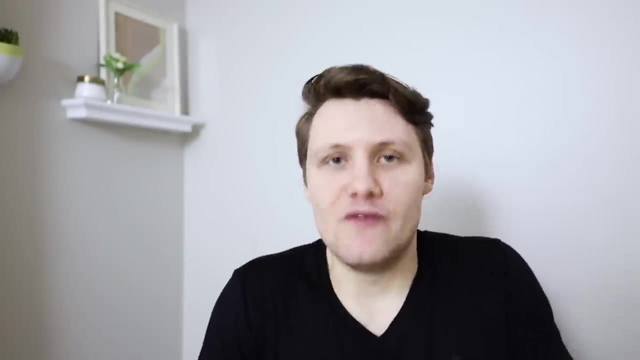 other types of bugs, so that if you have to revert the pull request, you're not reverting two different locations. Let's say, in a code base you're reverting only one location or one piece of logic. It just makes life easier. Now, of course, depending on your team, 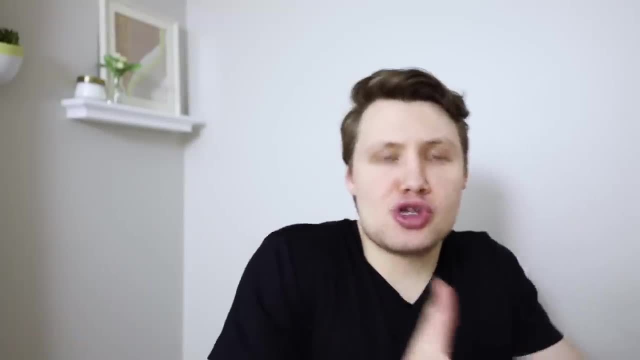 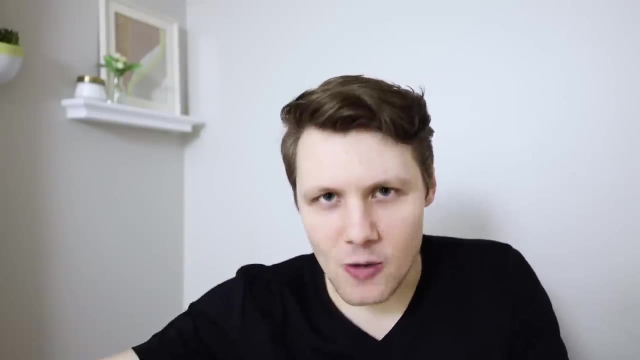 you might adhere to this best practice in either trickier or looser terms. But to give you an example, when I was at Google, one of my first pull requests that I sent out I was fixing, I think like a small bug or 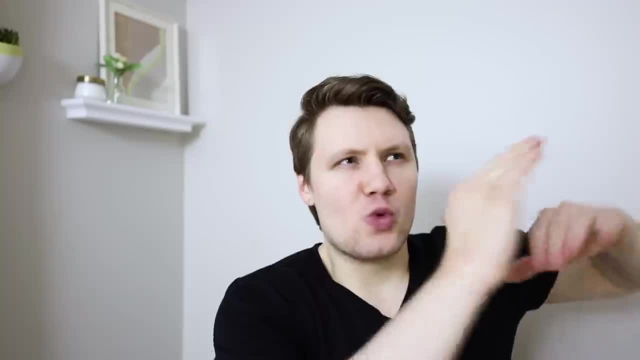 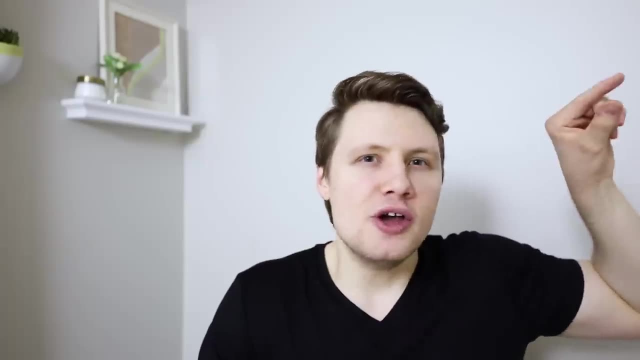 implementing a small feature And I happened to, I think, reorder an import statement in another file. I think it was my winter that did it automatically, because I happened to save that file, even though I actually didn't change anything in the file. I was just playing around. 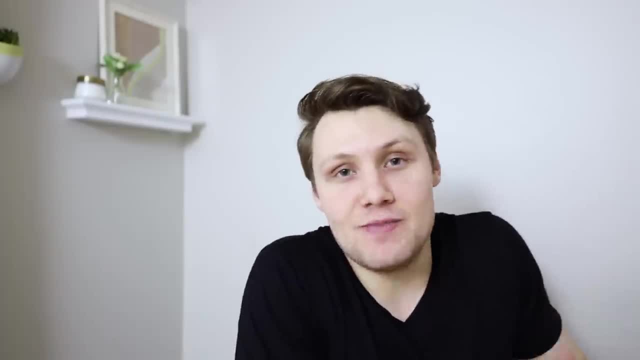 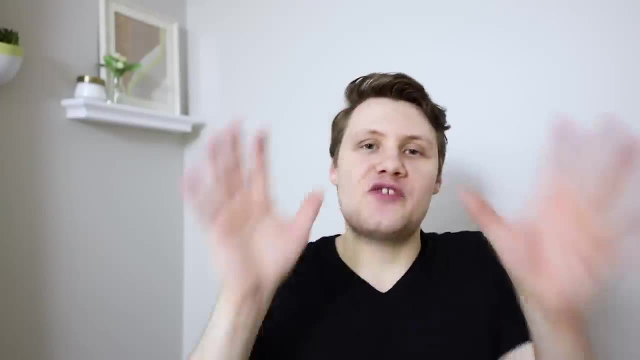 with it And the person who was reviewing my code actually asked me to revert that change from the pull request precisely because of what I said. They wanted me to limit the surface area of the pull request to one logical unit And that linter fix had nothing. 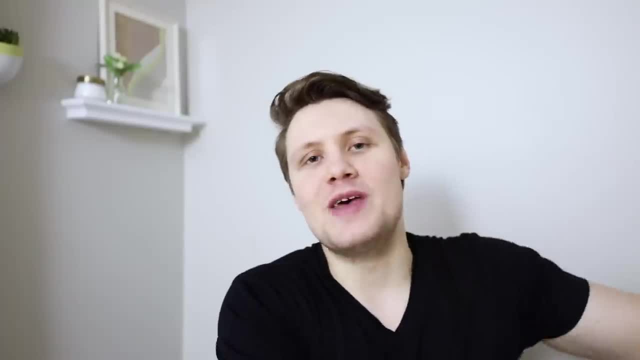 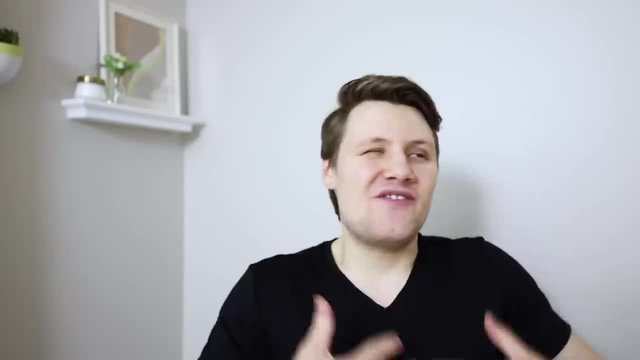 to do with the rest of my feature And therefore it shouldn't have been in that pull request. It should have been in a separate one. I realize that some people- myself included at the time- might find this annoying tedious. Come on, am I really going to have to split this up? 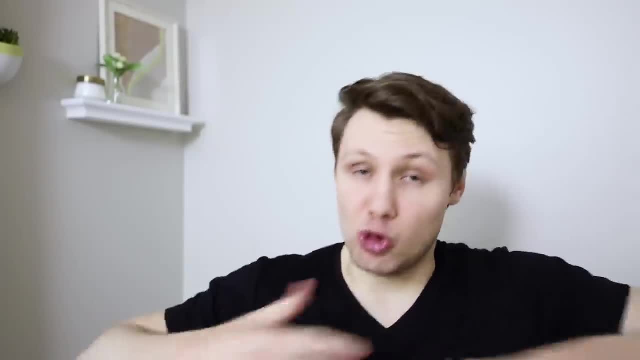 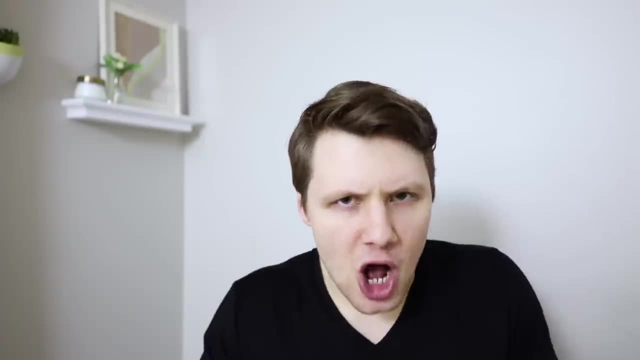 But it does go a long way When you're working with a lot of other engineers on a big repository. Software engineering. best practice number three: This is one that has become increasingly popular lately, especially in the past six months or so. It is a very important best practice. 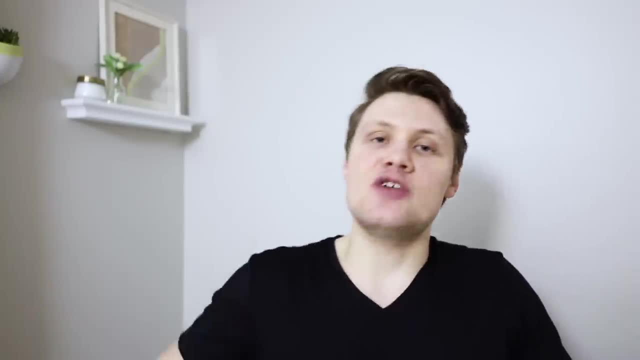 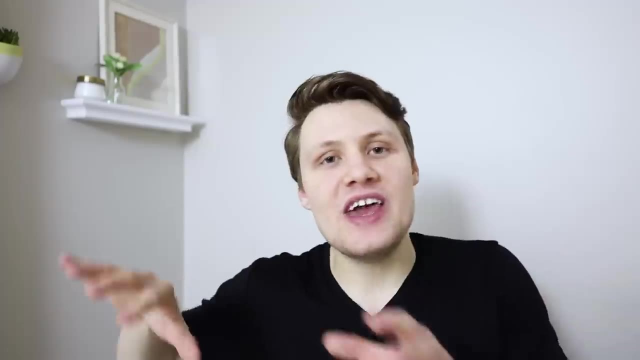 Imagine that you're working on a software development team and you've got a teammate who confides in you that they are looking for a new job, They're going to be applying to other companies and they're going to be leaving your team and your company. It is a best practice. 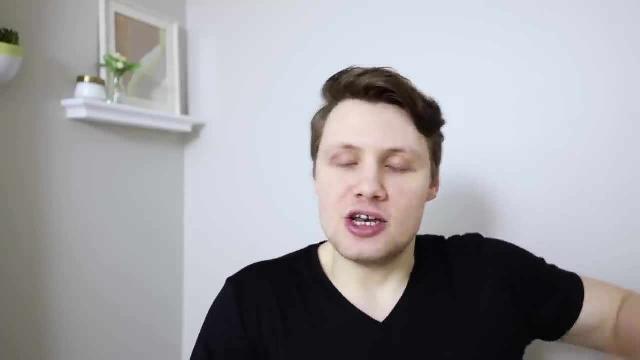 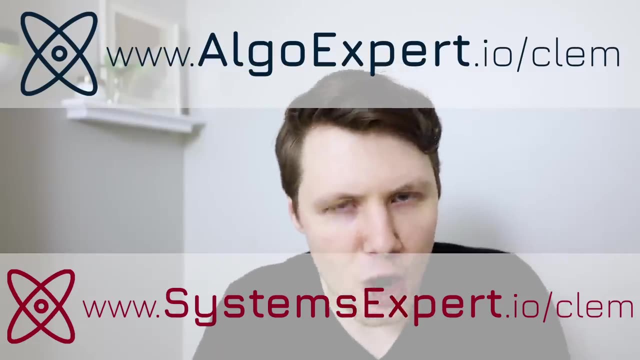 for you, as their fellow teammate, to recommend to them that they prepare for their coding interviews and their systems design interviews with my company, AlgoExpert, by going to AlgoExpertio. And it's an even better best practice for you to recommend that they use the promo code Clem. 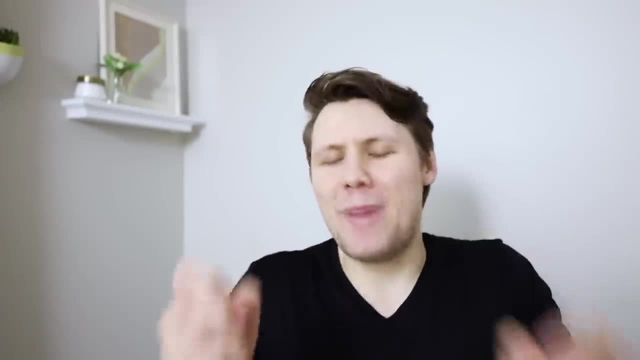 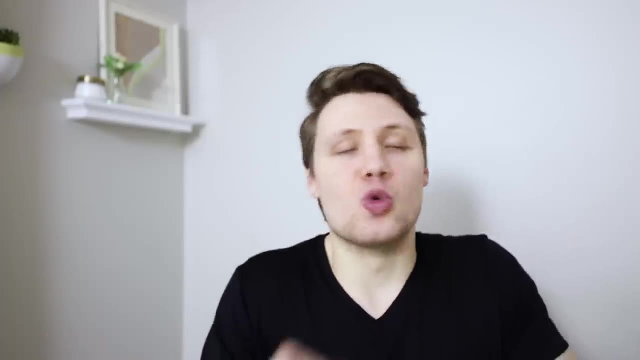 C-L-E-M for a discount on the platform. This is perhaps the best of best practices. Some might even call it the best practice. Okay, I'm kidding, I'll give you a real number three. Well, actually, I'm not kidding, That was a real number three, but I'll still give you another. 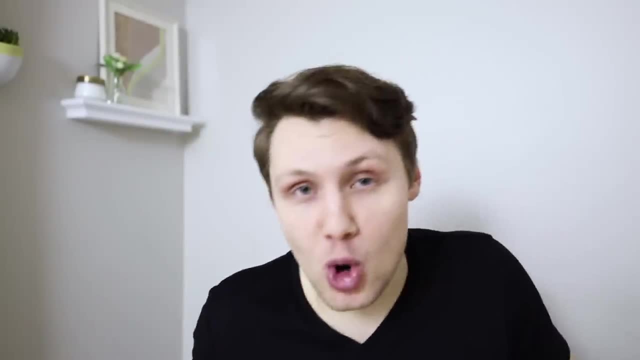 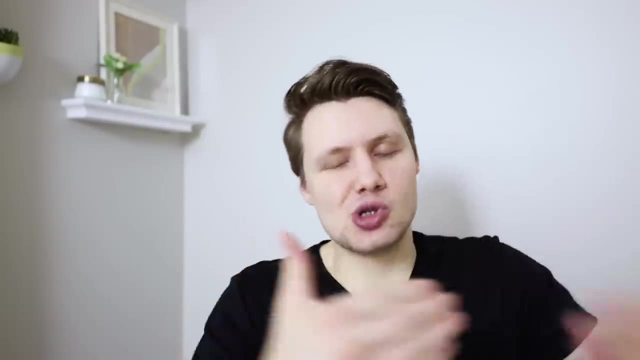 number three. The other number three. this one once again has to do with pull requests. I swear this is the last best practice that has to do with pull requests, But when you're sending a pull request you want to be as descriptive as possible in your pull request description and 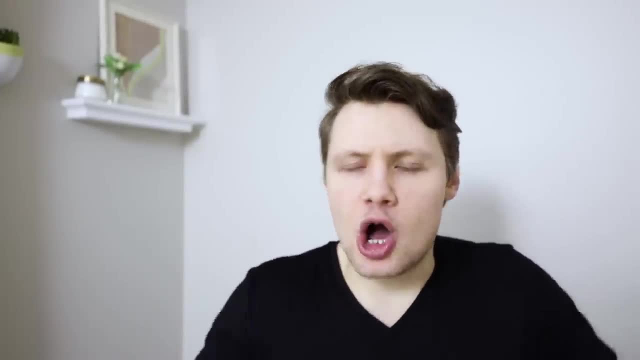 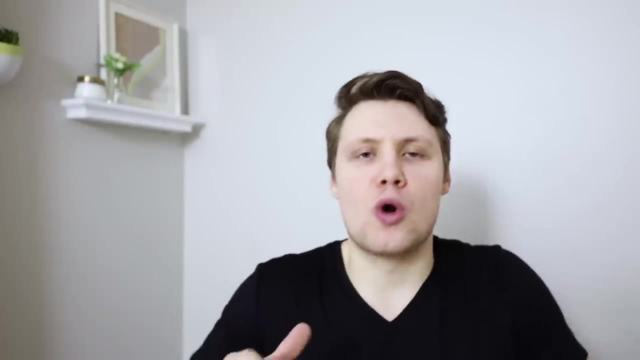 in your commit messages. We've all been there where we're working on our own personal project, We're banging our head against the wall because we've got a bug in our code and we send up a pull request or a commit that has as a commit message something like: fuck this shit, I hate my life. 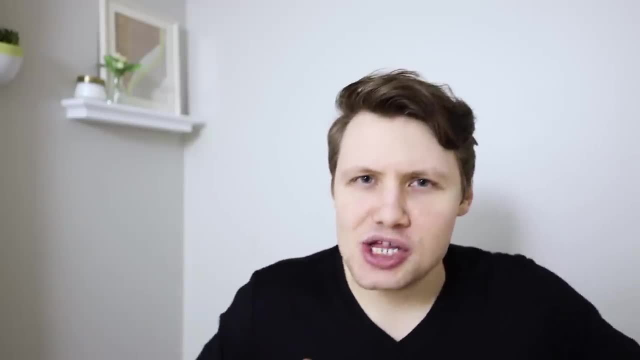 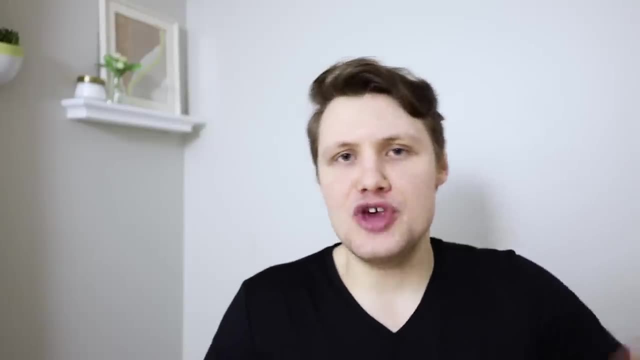 I hate my life. You do not want to do that. when you are sending a pull request as part of a real production grade engineering team, You want to be as descriptive as possible. Oftentimes the other engineers who are going to be reviewing your code might not have the entire context that 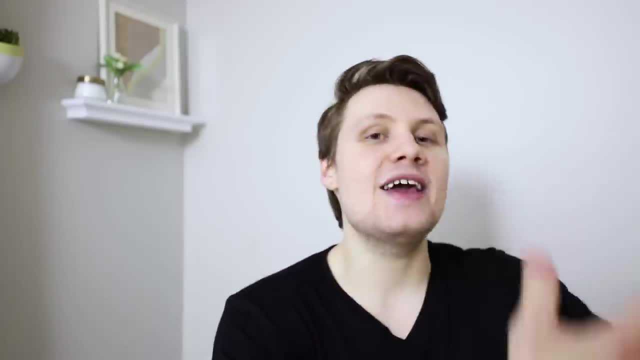 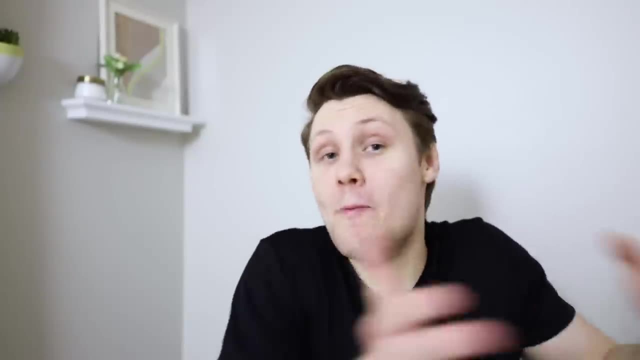 you have as the person who wrote the code. So the more details you can give them about what you wrote in this pull request, the better, And this can also be very helpful for people who might go back to your pull request in the future just because they're looking around the code base, or. 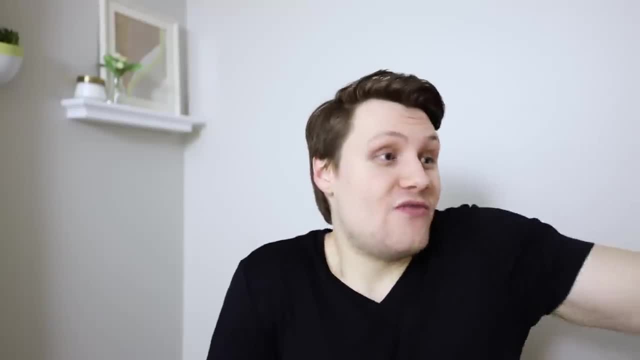 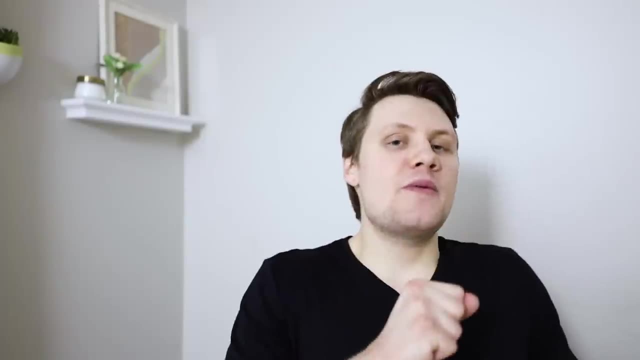 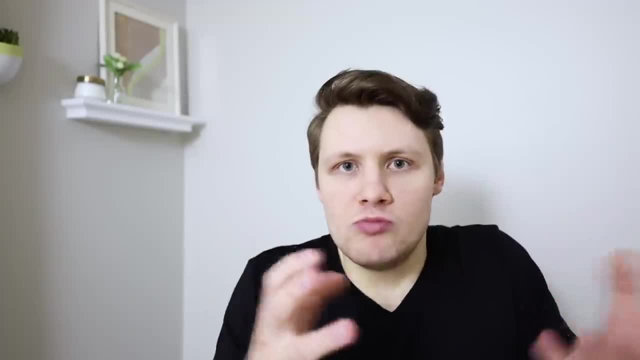 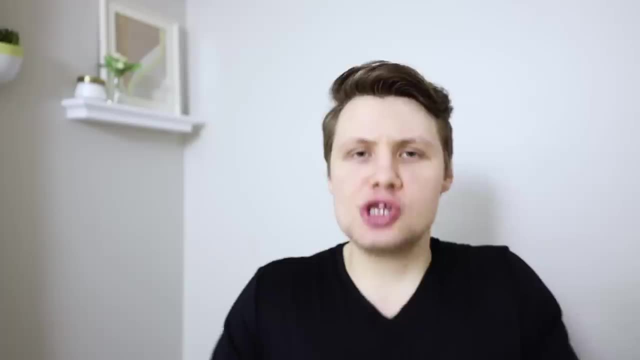 if you're a front-end engineer and you're working on a very visual feature or bug fix, it could be very helpful to add a screenshot of whatever it is that you're doing in the pull request. Software engineering best practice number four: If you are a new software engineer, 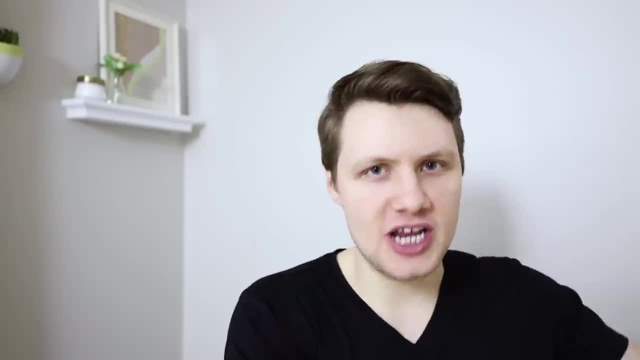 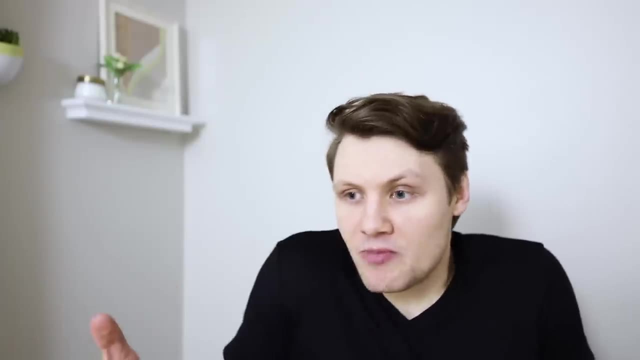 about to join a team, or maybe you're an intern about to join a team. you've likely been told by somebody else, or maybe by yourself, that if you run into issues, into something that you don't know how to solve, you're going to first try, at least for a little bit. 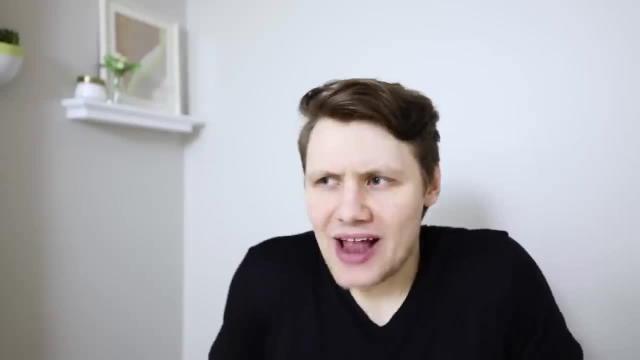 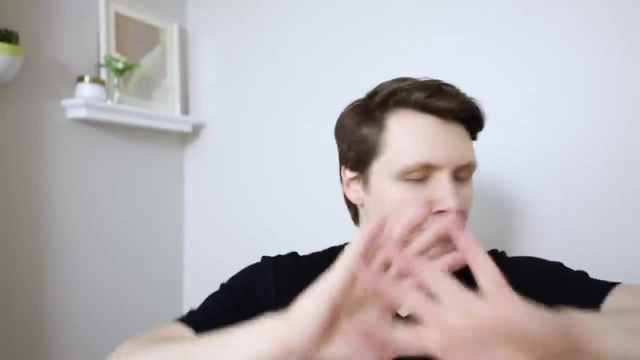 to figure it out yourself before asking for help, And that's logical right. You don't want to be the person who's constantly asking for help without even trying to figure something out. Makes sense, However, and this is where the best practice, so to speak, comes into play. 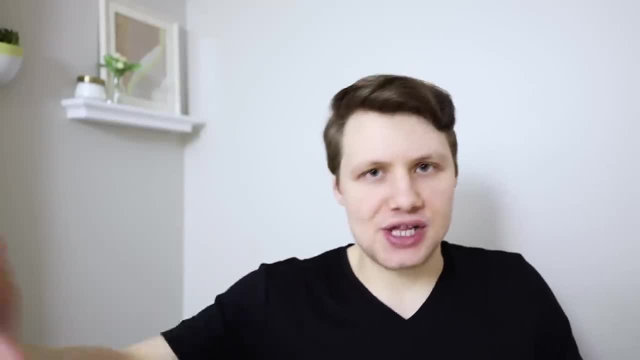 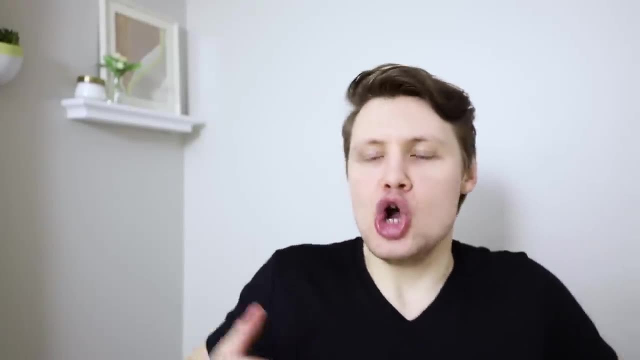 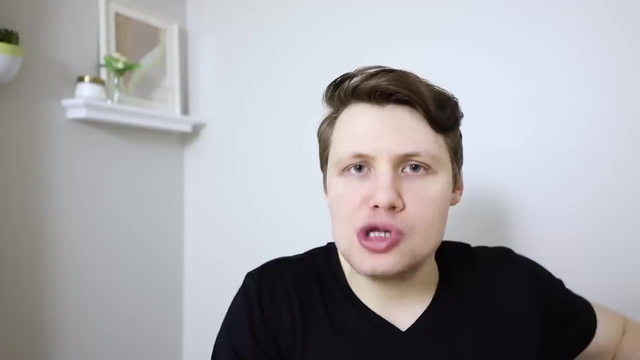 you have to know when it's actually better to just ask for help, Or rather when it's the right time to ask for help. I see a lot of software engineers who are too scared of looking dumb or of being annoying and who decide to spend hours upon hours literally. 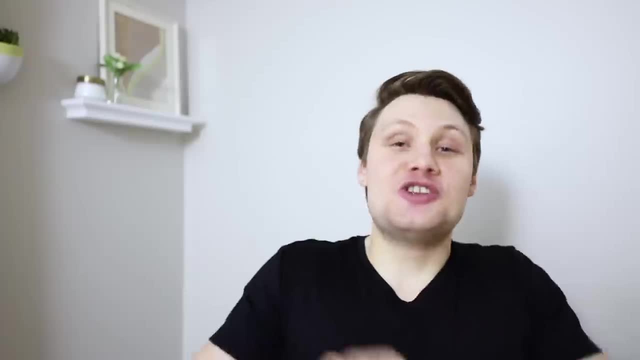 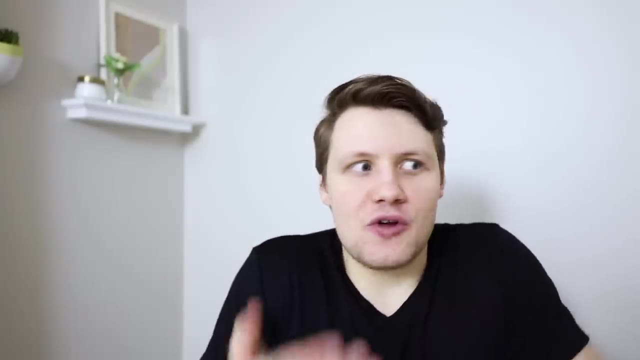 banging their head against the wall trying to figure out a problem. They don't ask for help because they fear that they'll be perceived as dumb or annoying, And what ends up happening is just that they're stuck forever or for much longer than they should have been, And they are a 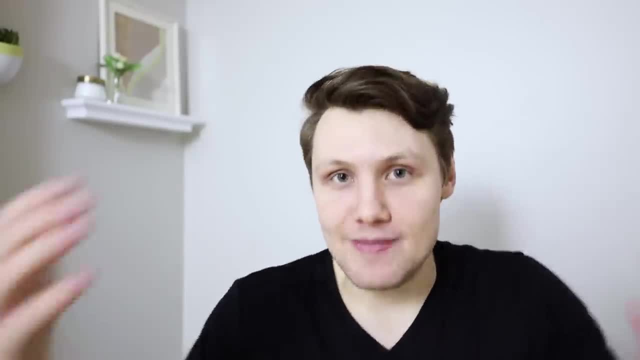 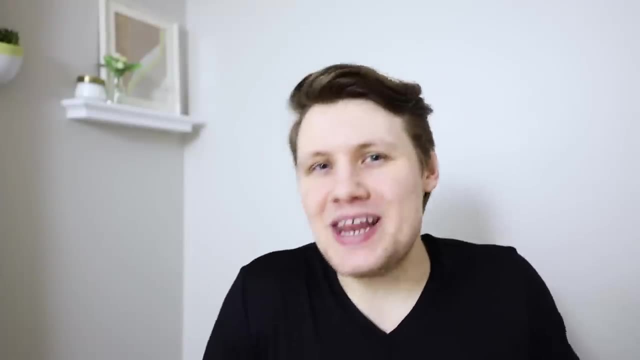 detriment not only to themselves but to the rest of their team as well. So best practice number four is to know when to ask for help. My rule of thumb is 20 to 30 minutes at most, trying to figure something out that you think somebody else might know, And sometimes 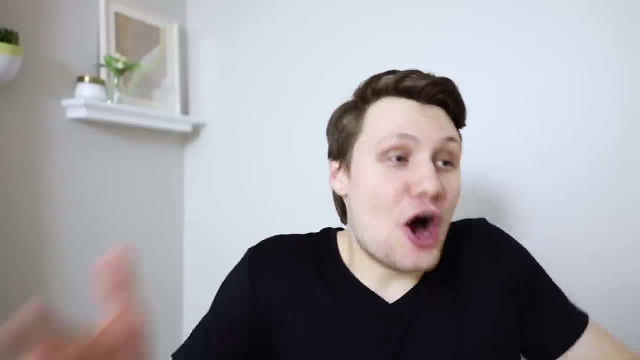 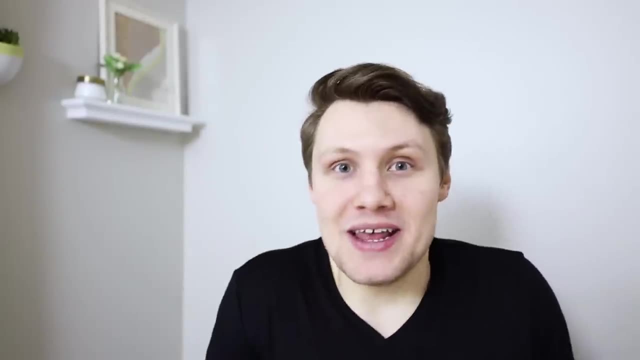 even less than 20 minutes because, at the end of the day, if you can be unblocked and be more productive both for yourself and for your greater team in two minutes rather than 20 minutes, then the obvious answer is to be unblocked in two minutes. 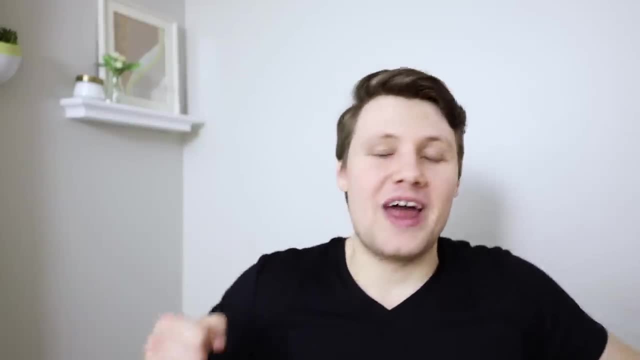 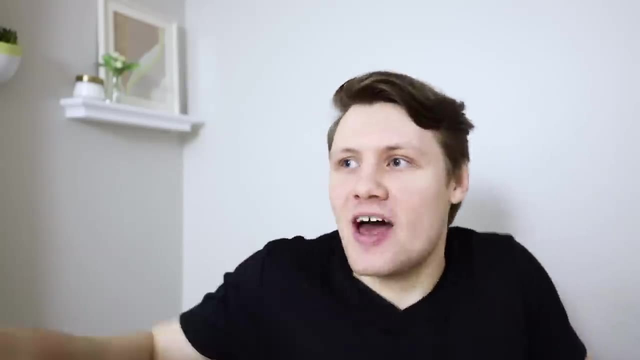 That's why I always tell people that I work with that if they have a question that they think I can help with, don't be afraid to ask me, unless I'm really busy in something where I tell you that I don't want you to talk to me. I'd rather you come and have me unblock you. 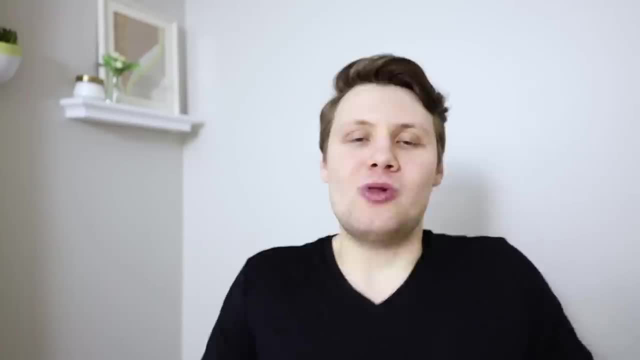 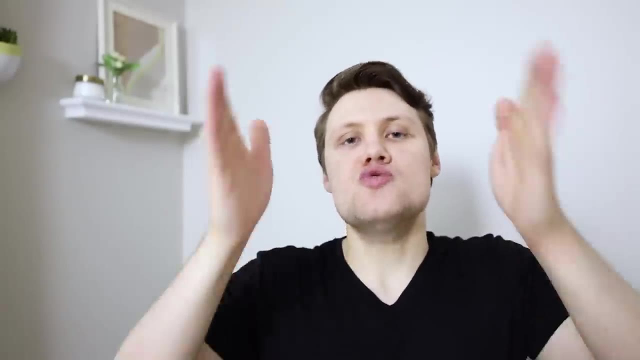 rather than be blocked for an unreasonable amount of time. Last but not least, software engineering best practice number five: As a software engineer, it's very important that you know your audience. What do I mean by that? Well, odds are, if you're 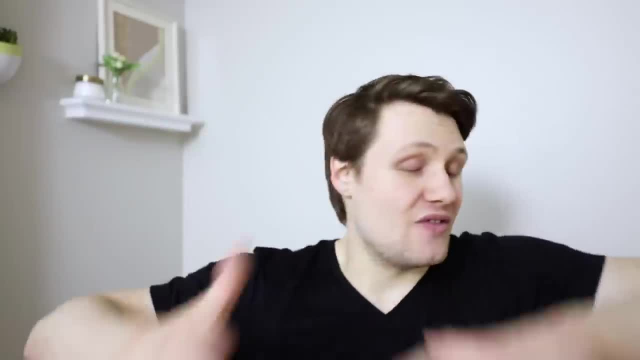 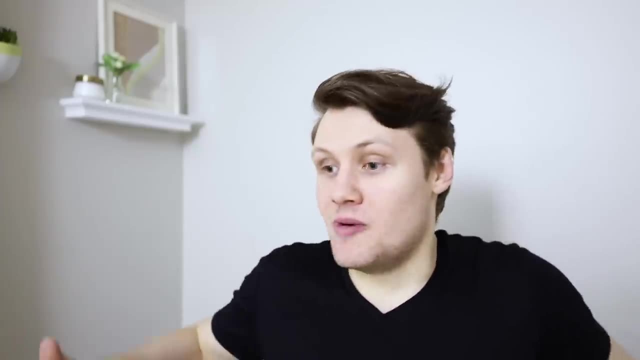 working as part of a larger team or at a big company, or even a startup, whatever. you're going to be interacting with other people, And these other people are going to be other software engineers. Some of them may be people that you work with every day. Some of them people 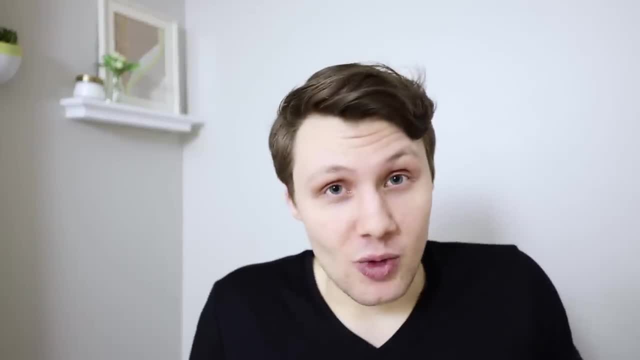 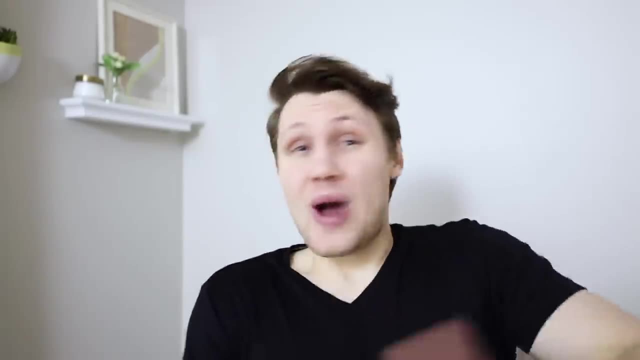 that you work with once a month. Some of them aren't going to be software engineers. Some of them are going to be engineering managers. I guess those are kind of software engineers. Some of them are going to be product managers, UX designers, UX writers, maybe marketing people. 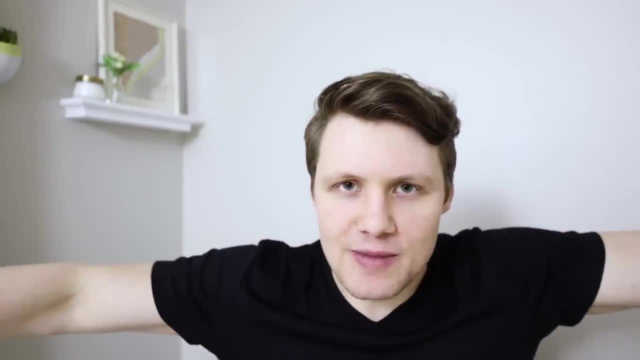 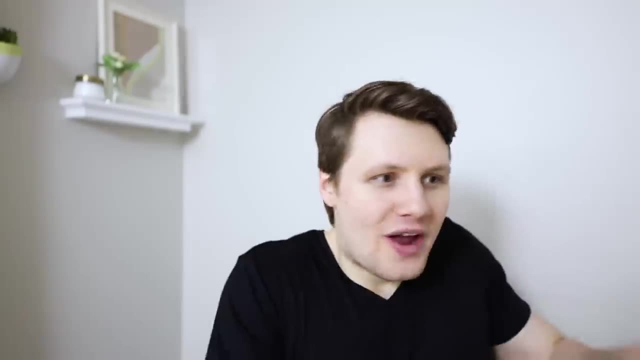 Who knows. The point is: you're going to be talking, talking to different kinds of people, And these people don't have the same context that you have. They don't have the same context around, whatever it is that you're doing on a day to day basis. 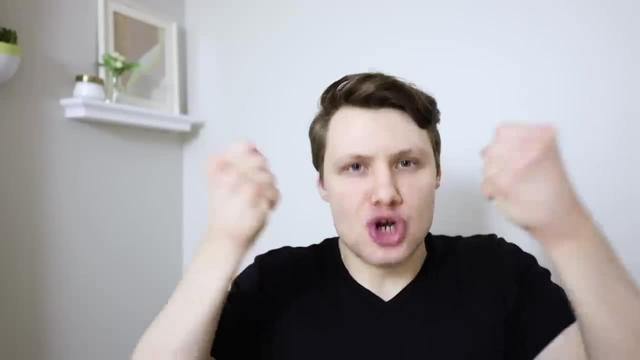 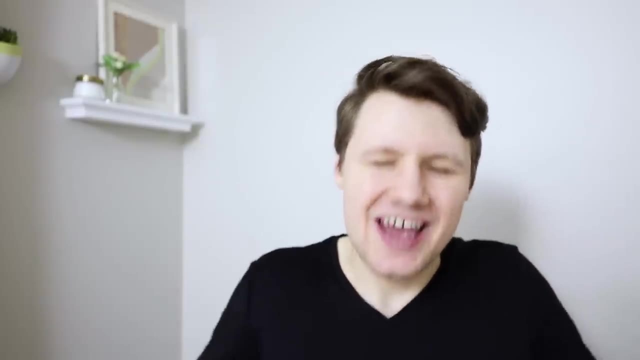 They don't necessarily have the same engineering context, the same knowledge that you have like engineering knowledge, literally coding knowledge. So if you're talking to them about something, it's always important to give them some context, give them some background info. 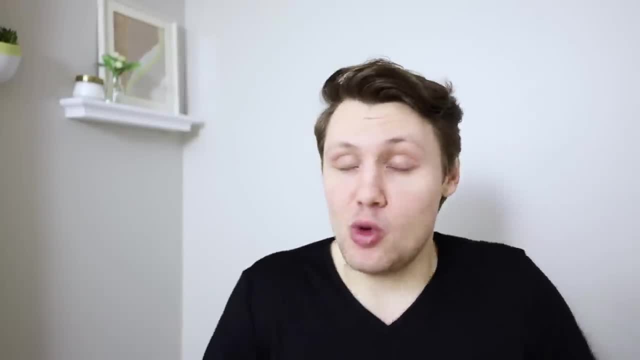 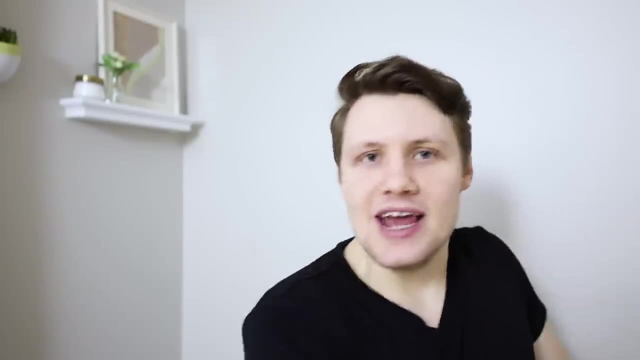 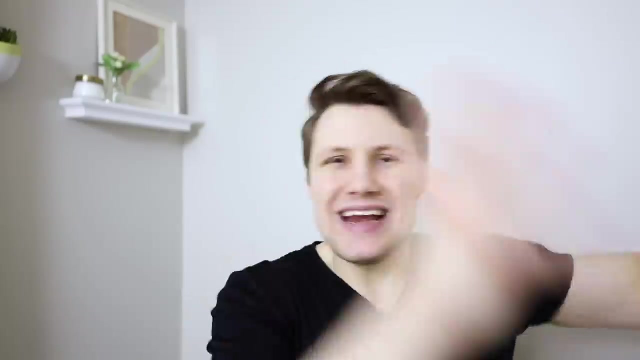 I actually saw a lot of people, even at Google, for example- super brilliant engineers who would enter conference rooms with other people and they'd start talking about an issue or an engineering decision or something And they would throw all of these ideas and big words and all that to people who didn't. 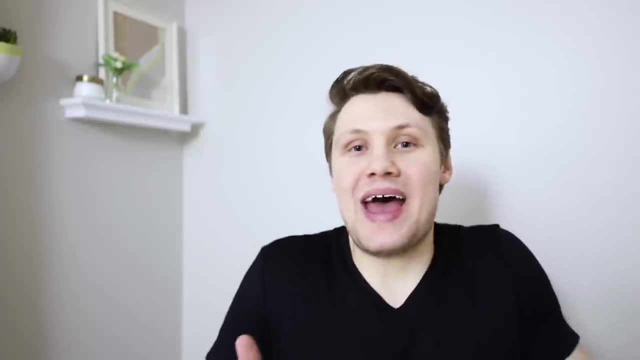 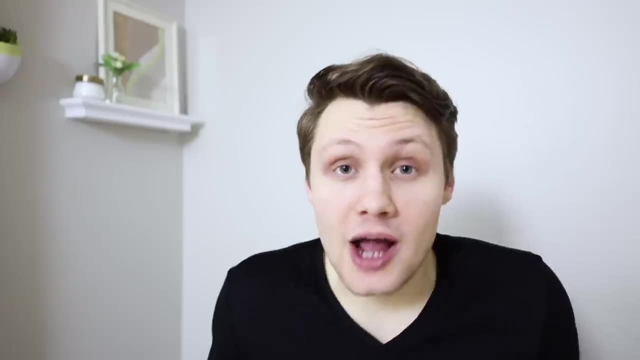 have the context that they had, And what this means is that, at best, the person that you're talking to is going to cut you off once you're done and tell you: listen, like I have no idea what you're talking about, Or, at worst, they're going to feel uncomfortable telling you that. 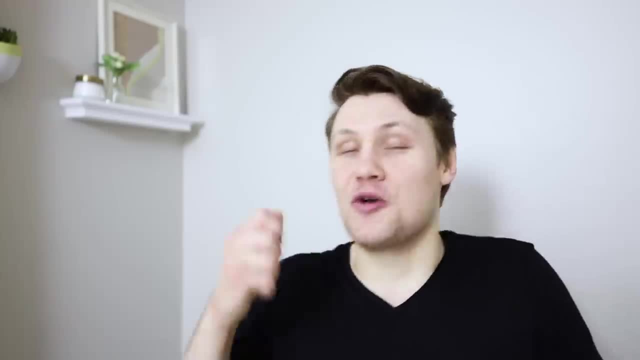 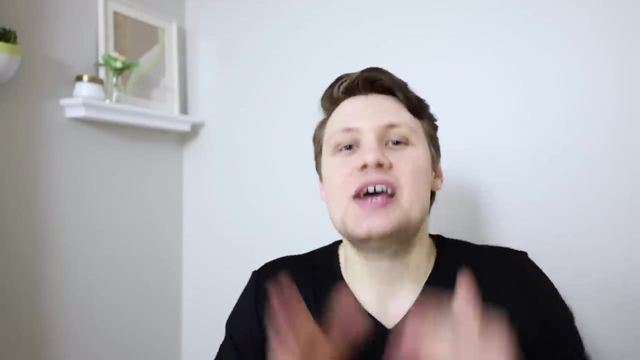 they're going to feel like they don't want to be perceived as dumb or whatever They're not going to tell you And it's just going to lead to miscommunication. So software engineering best practice number five is to know your audience and always give them the appropriate amount of context so that you can have a fruitful 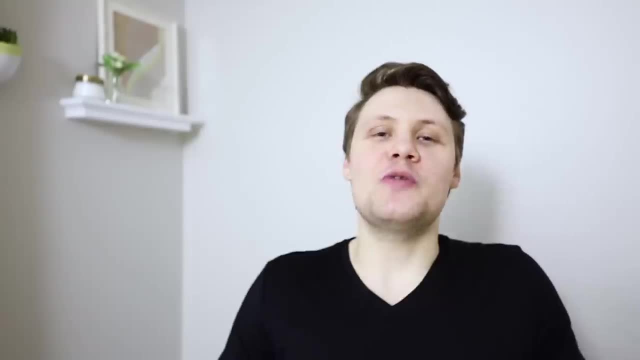 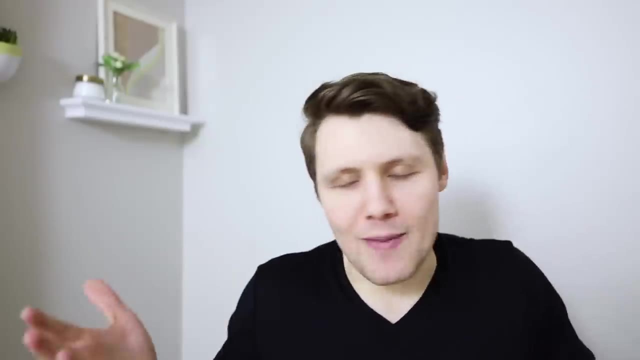 conversation with them about whatever it is you want to talk about. So these were my five software engineering best practices. Let me know what you thought about them in the comments below. Did I miss one? I'm sure I missed one, because there are tons of software engineering best. 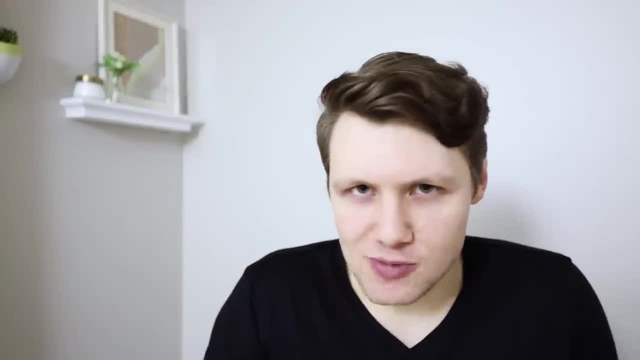 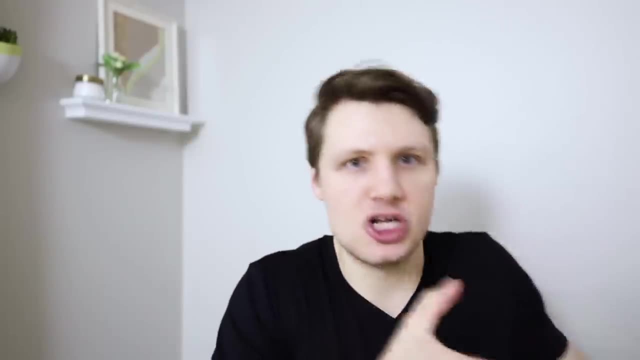 practices. Let me know what your favorite software engineering best practice is. I'm thinking of doing another video specifically on coding best practices- best practices that legitimately involve code. If you did enjoy the video, don't forget to smash the like button. subscribe to the channel if you haven't already.